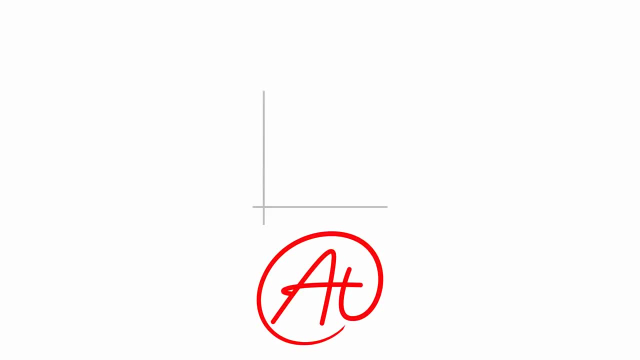 Hey guys, it's Mark from Ace Tutors And over the course of the next several videos I'm going to explain some of the most common probability distributions covered in statistics. In this video I'll go over the uniform distribution. So, first off, a uniform distribution is characterized by having a constant probability within a 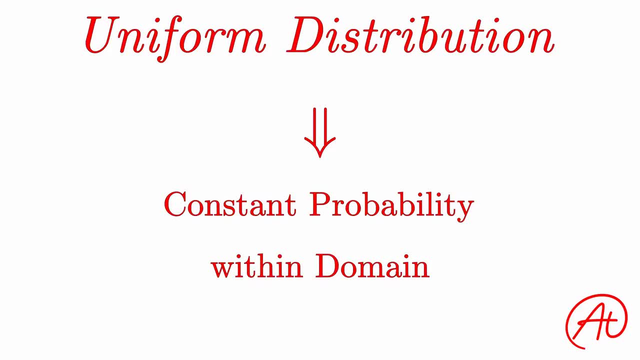 certain domain. But what does this mean? Well, to find out, let's take a look at this distribution on a graph where the x-axis represents the different values this certain event can be, while the y-axis represents the probability of those events. From this graph, you can: 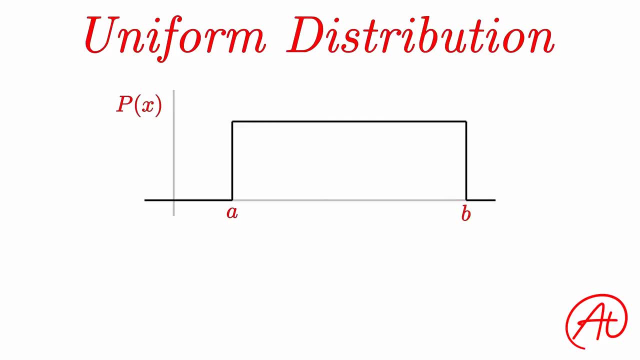 hopefully see how each x-value within the domain of A to B has the exact same y-value, which implies the same exact probability. But what is this constant probability? Well, we already know that if we add up all the probabilities of all the outcomes of a certain 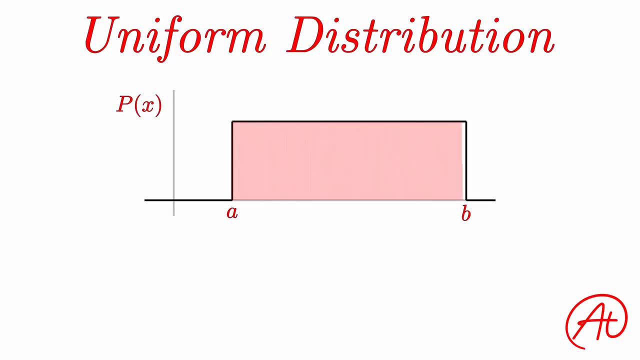 event, or in other words find the total area. under any probability distribution, the result must equal 1.. Since this area is a nice and simple rectangle, we can find its area by multiplying its height by its width. The width is simply found by subtracting B minus A. 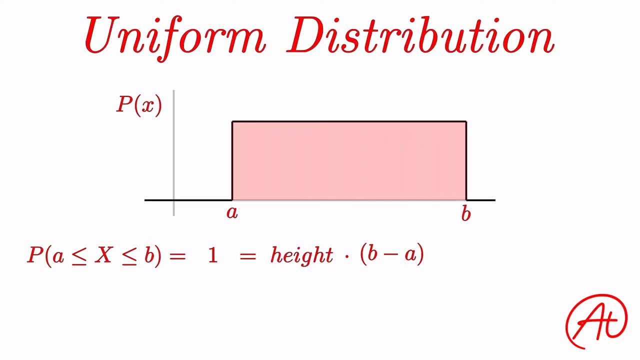 and now we can solve this equation. for what the height must be? Dividing both sides by B minus A, we get that the height of this distribution must be 1 over B minus A. Okay, now that we covered the general look of the uniform distribution, let's go over. 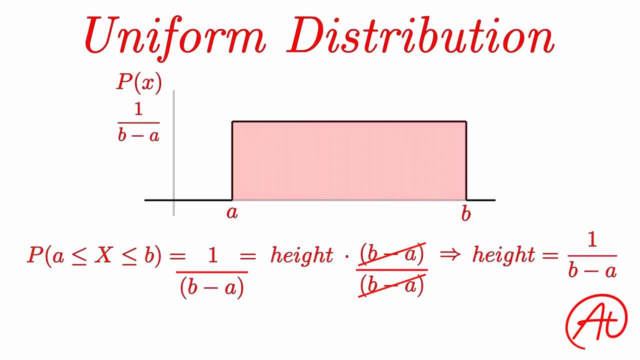 some common values associated with this distribution. First, let's find its mean or expected value, Because the distribution is nice and symmetric. the mean mu ends up being right in the middle of its domain, which you can find by taking the average of the domain bounds, aka A plus. 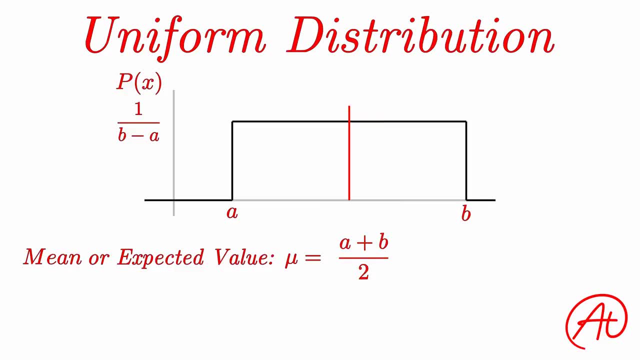 B divided by 2.. And once again from the distribution symmetry, this value ends up being the same for the median. Okay, moving on to standard deviation, this formula ends up being a little less intuitive For a uniform distribution. the standard deviation sigma ends up being the square root of B minus. 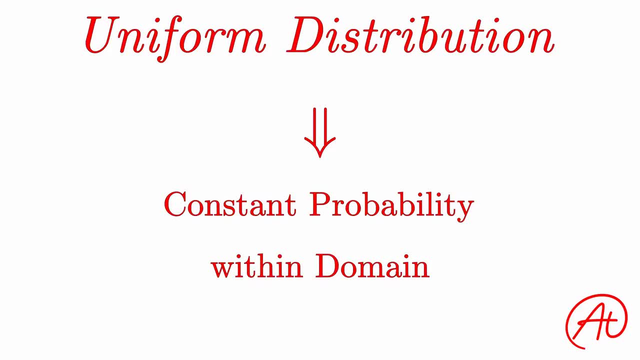 certain domain. But what does this mean? Well, to find out, let's take a look at this distribution on a graph where the x-axis represents the different values this certain event can be, while the y-axis represents the probability of those events. From this graph, you can: 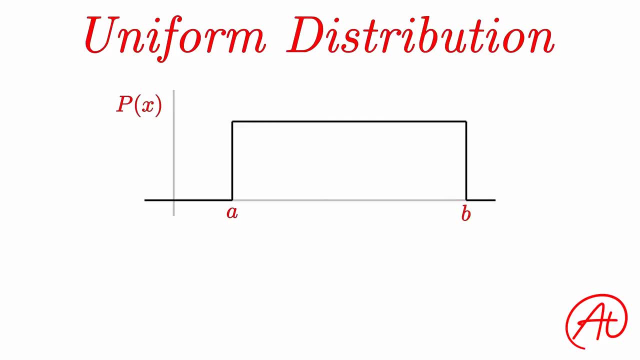 hopefully see how each x-value within the domain of A to B has the exact same y-value, which implies the same exact probability. But what is this constant probability? Well, we already know that if we add up all the probabilities of all the outcomes of a certain 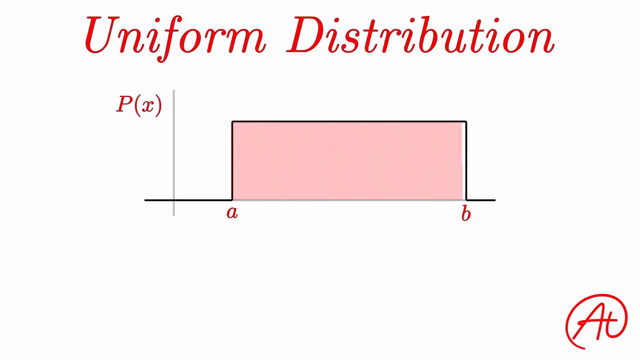 event, or in other words find the total area. under any probability distribution, the result must equal 1.. Since this area is a nice and simple rectangle, we can find its area by multiplying its height by its width. The width is simply found by subtracting B. 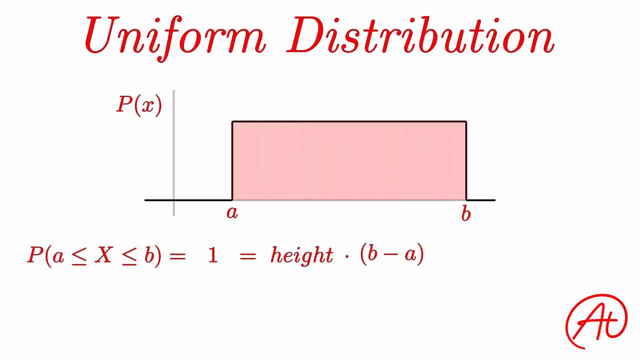 minus A. and now we can solve this equation. for what the height must be? Dividing both sides by B minus A, we get that the height of this distribution must be 1 over B minus A. OK, now that we covered the general look of the uniform distribution, let's go over 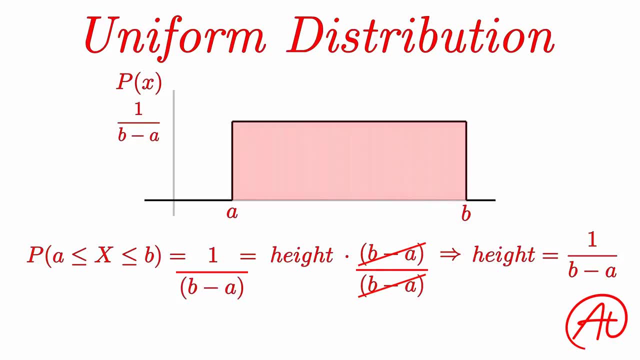 some common values associated with this distribution. First, let's find its mean or expected value, Because the distribution is nice and symmetric. the mean mu ends up being right in the middle of its domain, which you can find by taking the average of the domain bounds, aka A plus. 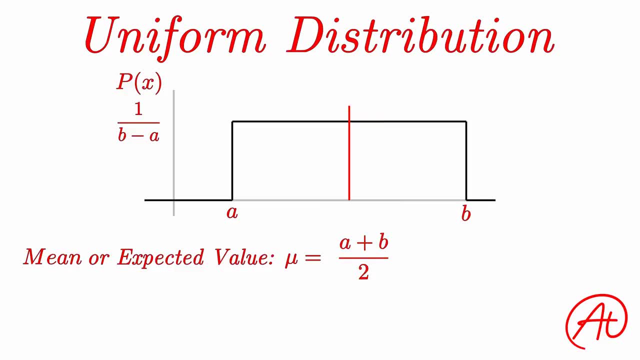 B divided by 2.. And once again from the distribution's symmetry, this value ends up being the same for the median. OK. moving on to standard deviation, this formula ends up being a little less intuitive For a uniform distribution. the standard deviation sigma ends up being the square root of B minus. 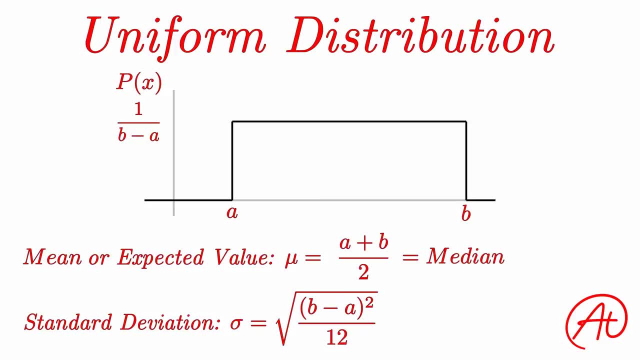 A squared divided by 12.. Next, let's go over some of the fun stuff: probability. When we discuss finding probability for continuous functions like this, we generally want to find the probability of a range of things occurring. For example, we might want to find: 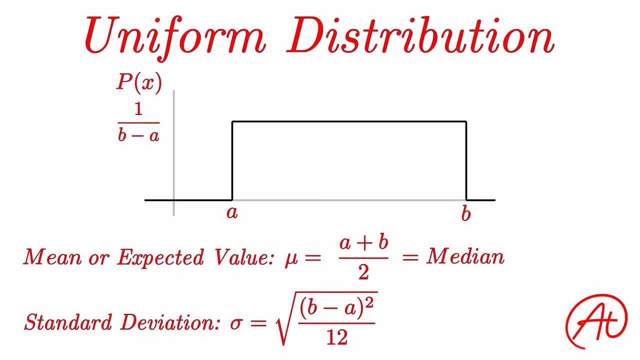 A squared divided by 12.. Next, let's go over some of the fun stuff: probability. When we discuss finding probability for continuous functions like this, we generally want to find the probability of a range of things occurring. For example, we might want to find: 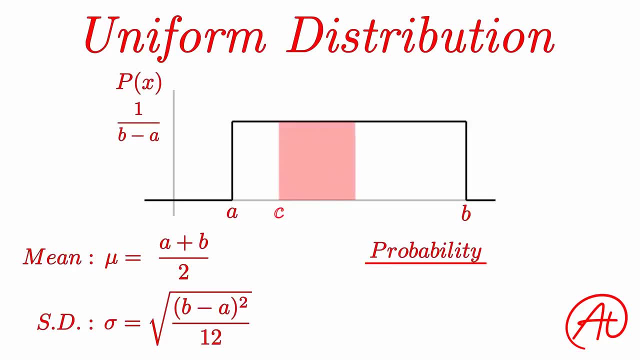 the probability of our event's outcome being between C and D. To calculate this, we could approach it one of two ways. You can either see it as a rectangle and calculate the area by LXW, Or understanding that the distribution is uniform. you can find Constitution isısıxf, 3² over εx, which you can substitute Pا by 1 over KT. 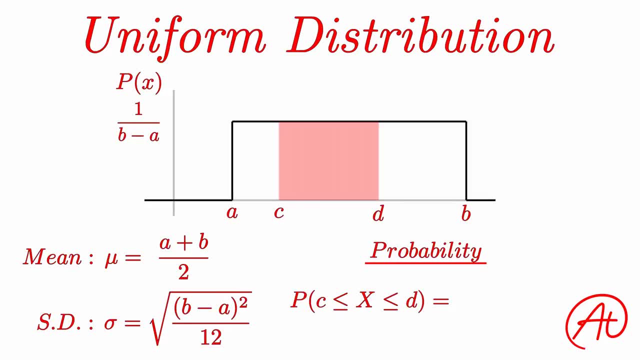 That's something cute. you can find the fraction that the desired interval makes up the entire distribution's domain. Either way, you would end up with the same result of d minus c divided by b minus a. Now that we covered some general terms from the uniform distribution. 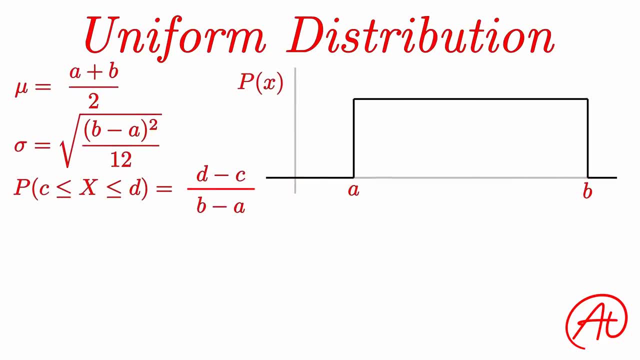 let's put the theoretical garbage aside and see how this works with a concrete example. Say that you take the bus to work and every day the bus is uniformly late- between 2 and 10 minutes On any given day. how long can you expect to wait And with what standard deviation? 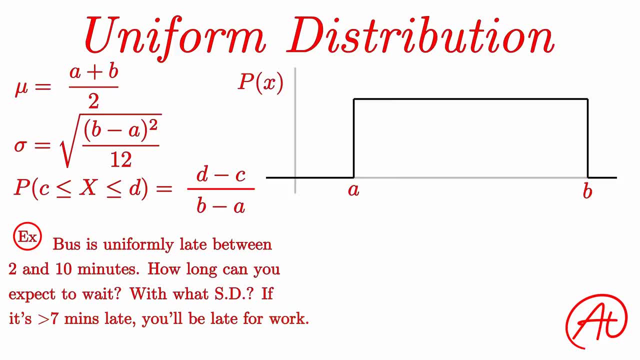 Finally, if the bus is late more than 7 minutes, you'll be late to work. So what is the probability that you'll be late on any given day? Okay, first let's set up our graph. Instead of a and b, we can replace these values. 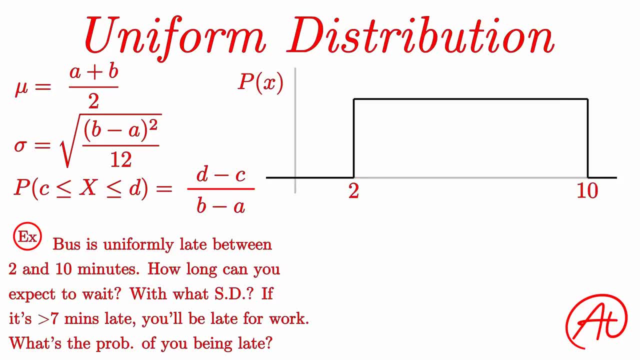 We have 2 and 10, because that's the entire domain for the bus's arrival time. Now let's start solving some of these questions. First, we want to find how long we can expect to wait for the bus on any given day. 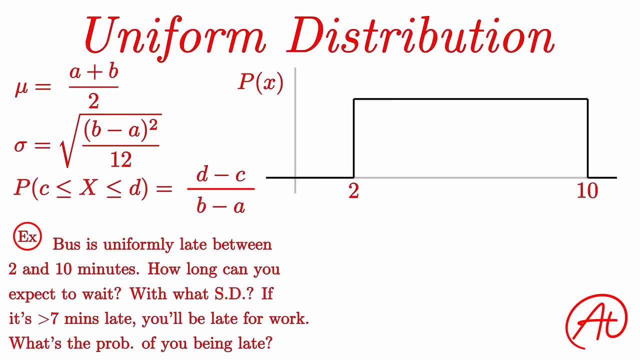 Well, this is a job for the expected value formula. We can calculate mu by finding the middle of the domain, which is 12 over 2, or 6.. And since this is a word problem, we have to add in our units. 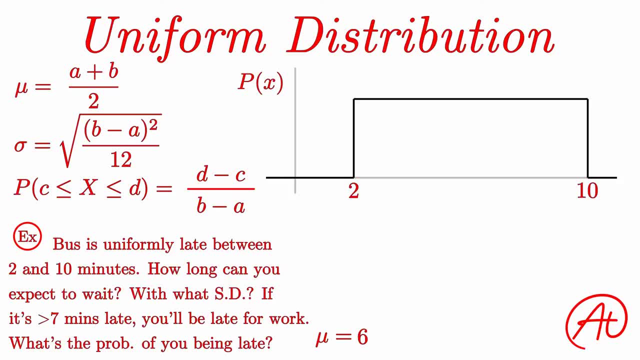 Because of the units in the question, we find that we can wait an average of 6 minutes on any given day. Next, we want to calculate the standard deviation of our wait times. Using our standard deviation formula, we find that sigma is equal to the square root of 64 over 12, or about 5.33.. 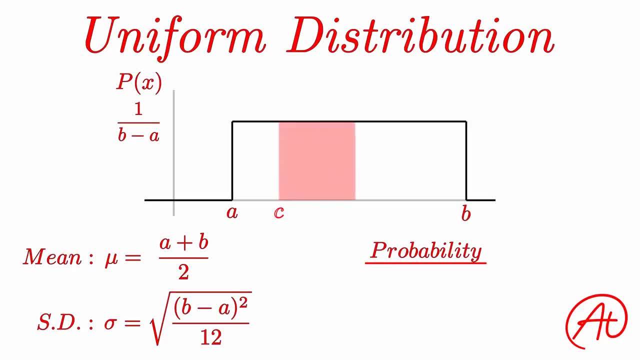 the probability of our event's outcome being between C and D. To calculate this, we could approach it one of two ways. You can either see it as a rectangle and calculate the area by length times width, Or understanding that the distribution is uniform. you can find: 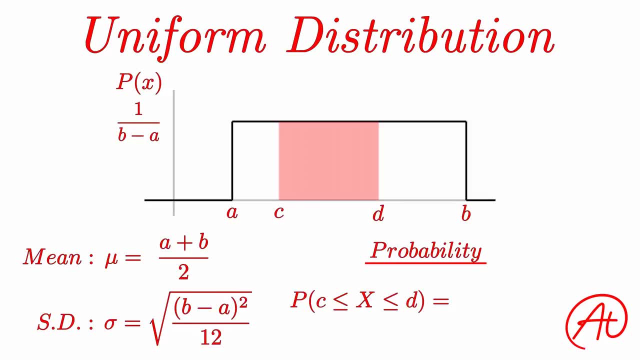 the fraction that the desired interval makes up the entire distribution's domain. Either way, you would end up with the same result of D minus C divided by B minus A. Now that we covered some general terms from the uniform distribution, let's put the theoretical. 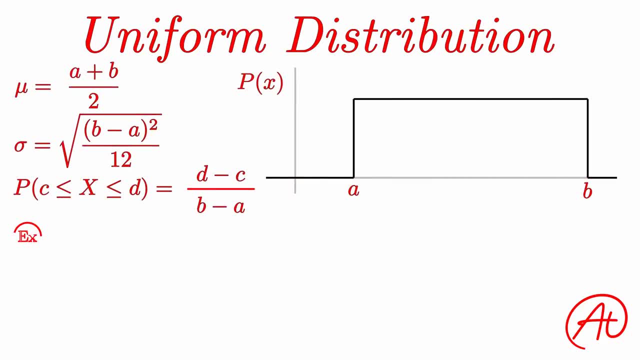 garbage aside and see how this works with a concrete example. Say that you take the bus to work and every day the bus is uniformly late- between two and ten minutes On any given day. how long can you expect to wait, And with what standard? 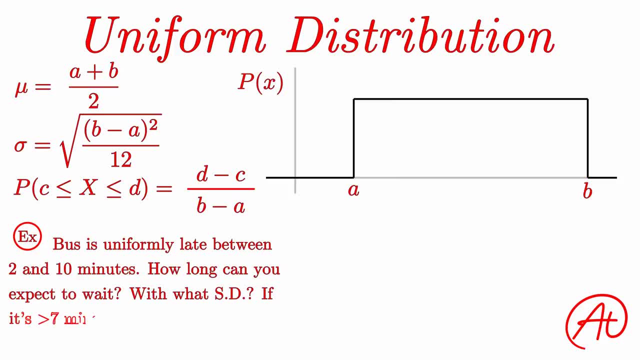 deviation. Finally, if the bus is late more than seven minutes, you'll be late to work. So what is the probability that you'll be late on any given day? Okay, first let's set up our graph. Instead of A and B, we can replace these values with: 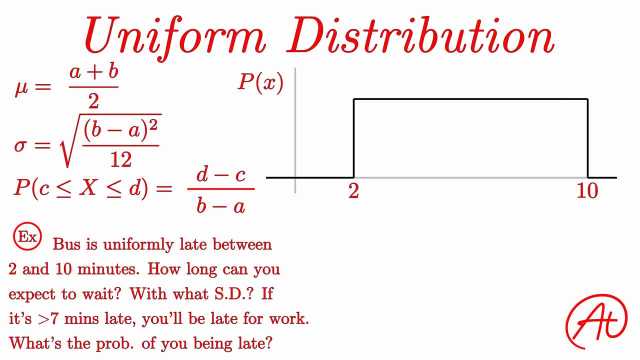 two and ten, because that's the entire domain for the bus's arrival time. Now let's start solving some of these questions. First, we want to find how long we can expect to wait for the bus on any given day. Well, this is a job for the expected value formula We can. 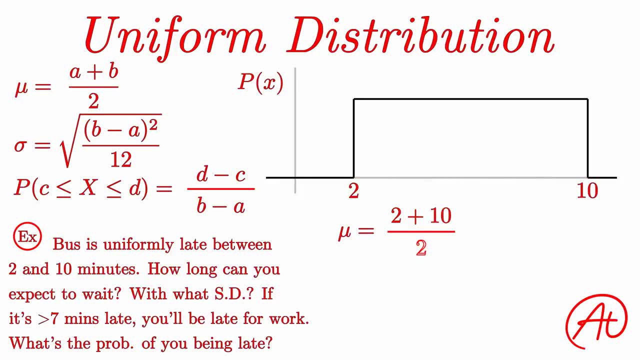 calculate mu by finding the middle of the domain, which is twelve over two or six. And since this is a word problem, we have to add in our units. Because of the units in the question, we find that we can wait an average of six minutes on any given day. 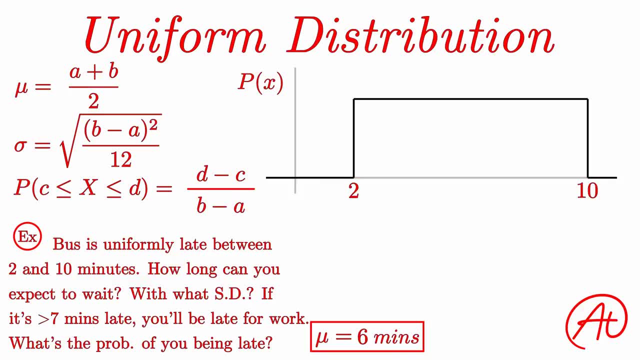 Okay. Next, we want to calculate the standard deviation of our wait times. Using our standard deviation formula, we find that sigma is equal to the square root of sixty-four over twelve, or about five point three three, And what this represents is that the wait times deviate. 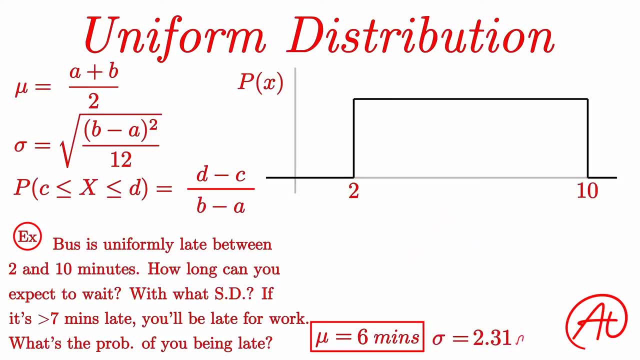 from the mean on average, an amount of two point three, one minutes. Finally, in order to calculate the probability of being late to work, we essentially need to find the probability of the bus being over seven minutes late. Since the bus's arrival time has an upper bound of ten minutes late, we need to find the probability of it being 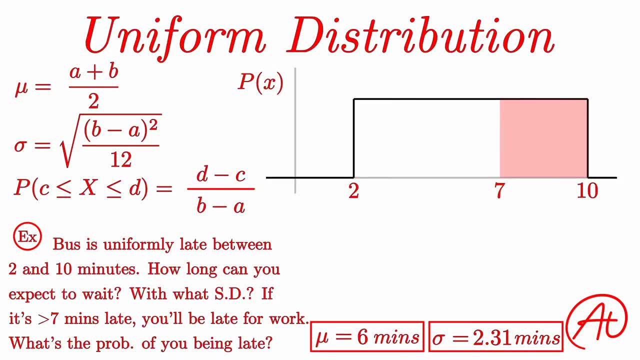 between seven and ten minutes. Using our probability formula, we find that this probability ends up being three over eight, or point three, seven, five. So that's the basics of the uniform distribution. In future videos I'll be talking about the distribution of the bus and how to calculate the probability of the bus being over seven. 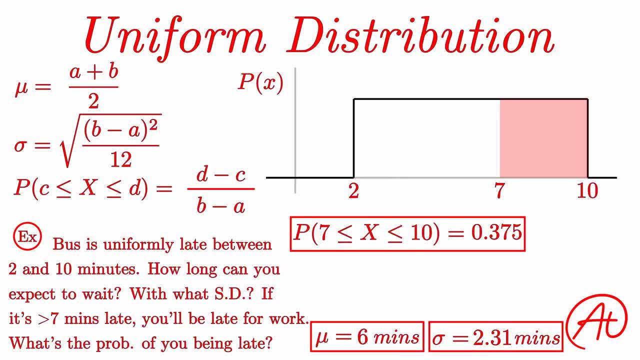 minutes late, I'll be explaining some of the more complex distributions that you'll come across in your class. For now, if you have any additional topics or videos you want to see made, please let us know down in the comments. And, as always, if you found this video helpful, please consider giving us a thumbs up and. 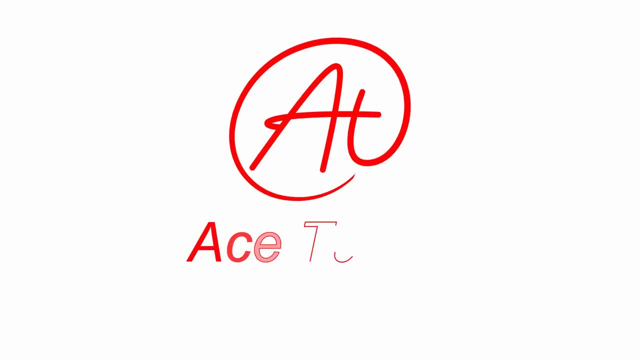 subscribing to our channel. Thanks again for watching and remember you have big dreams. don't let a class get in the way. I'll see you in the next video. Hi, in this video we're going to talk about solving very basic trigonometric equations. So, what makes trigonometric equations unique when you compare them to other types of equations, the periodic behavior of every single trigonometric function creates multiple solutions. 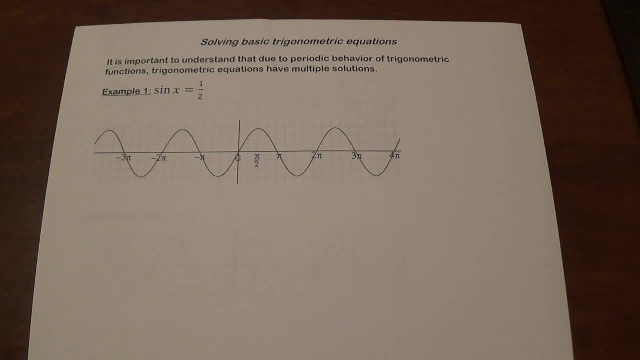 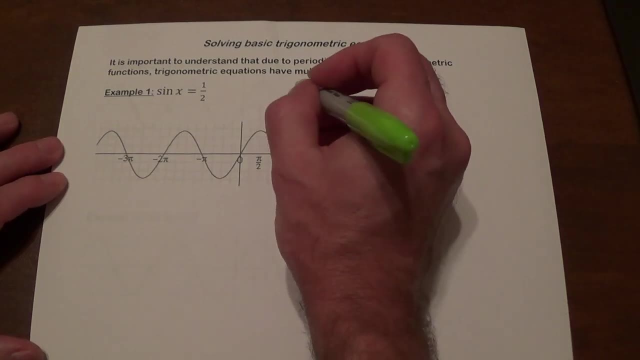 So, let's go ahead and start with this problem, sine x equals 1 half. So, where is that going to happen? Well, if you think about the unit's circle, we know that's going to happen when the angle is pi over 6, right? 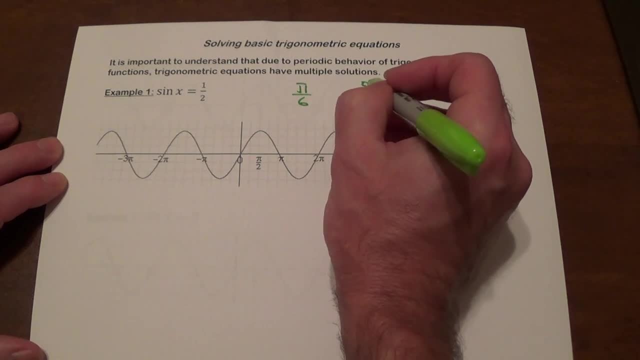 And we also know it's going to happen when the angle is 5 pi over 6. Then these functions are going to have a period of 2 pi, right?